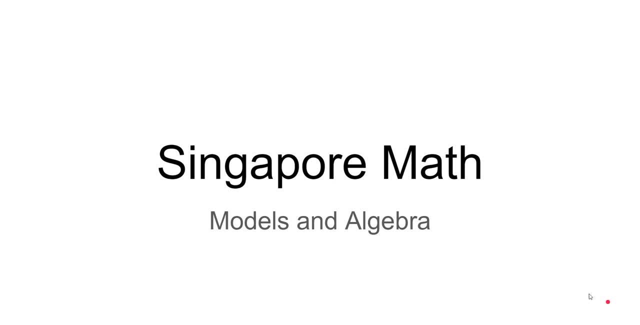 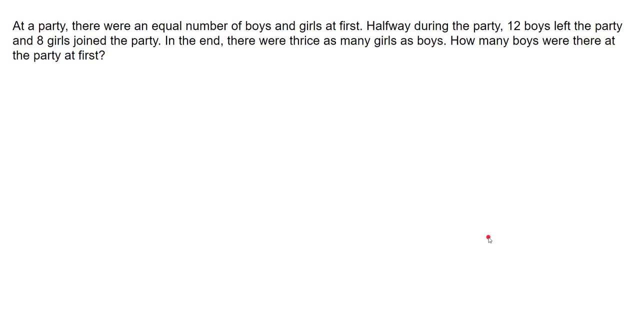 Hi everyone. today we are going to solve another word problem using Singapore math models and also you solve the problem using algebra. Let's dive straight into the problem. At a party there were an equal number of boys and girls. at first Halfway during the party, 12 boys left and 8 girls joined In the 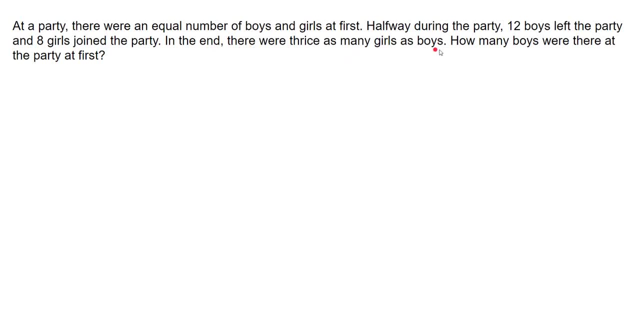 end, there were thrice as many girls as boys. What this statement tells you is that the number of girls were three times the number of boys at the end of the party. How many boys were there at the party at first? So we can actually. 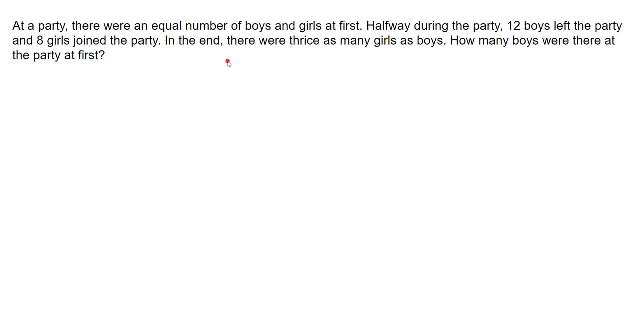 when you look at this question. there are three distinct set of information that you can look at. One is before, at the beginning of the party, the number of boys and girls were equal. Second, there is a change in the middle of the party: 12 boys left and 8 girls. 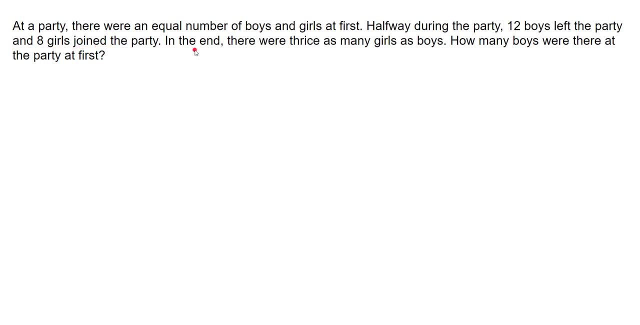 joined. So at the end, what happens? there will be 12 less boys and 8 more girls, and now the number of girls become three times the number of boys. So then we are asked to find out the number of boys at the party at first. So we go ahead and 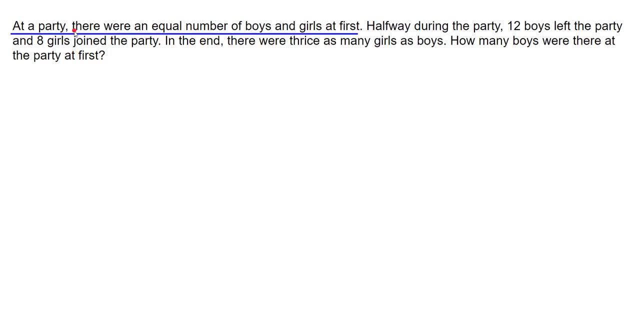 take the first information: At the party there were an equal number of boys and girls at first. So let's say boys, we draw a model for boys. This represents the total number of boys at the party in the beginning and girls- there were an equal number of girls, so girls will also have the same. 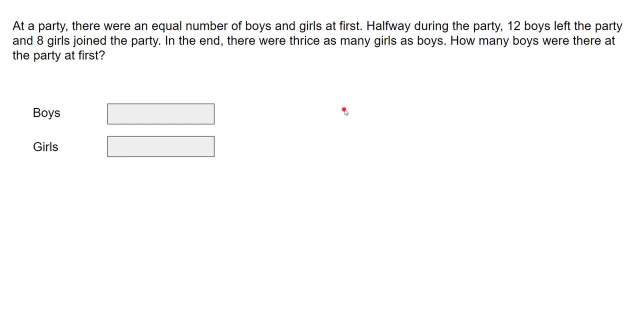 sized model diagram that you see here. Then what happens? halfway during the party? 12 boys left the party And 8 girls joined. So this 12 is gone, 12 boys. We are just arbitrarily taking some size here and saying this 12 is gone and 8 girls joined the party. So additionally there. 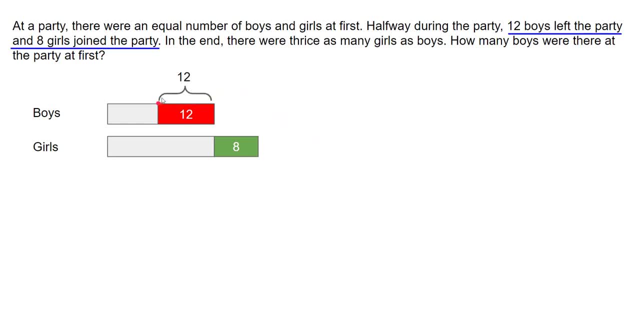 is an 8 added here, So we are just going to mark this out, because this is going to be gone away. So we just want to know that the size of this is actually a constant number, 12.. And 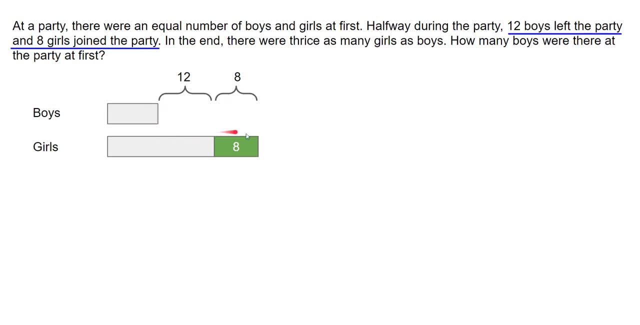 Yes, you can see already it wasn't a constant number: 12. there was an texted number at the beginning of the day and there was another 7 here, now that the number 12 it was. 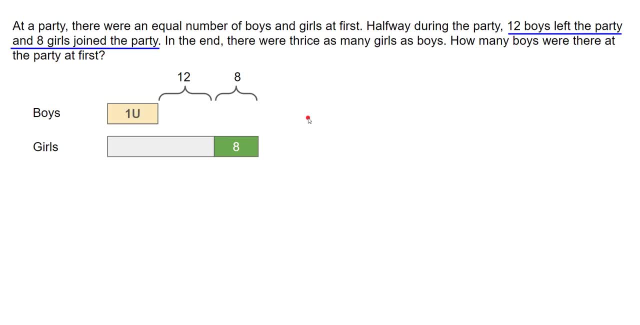 This is 8 here. So this whole thing from here to here, we know is actually made of 12 students and 8 students here. Now, at the end, what happened in the end? they were thrice or three times as many girls as boys, or the number of girls was three. 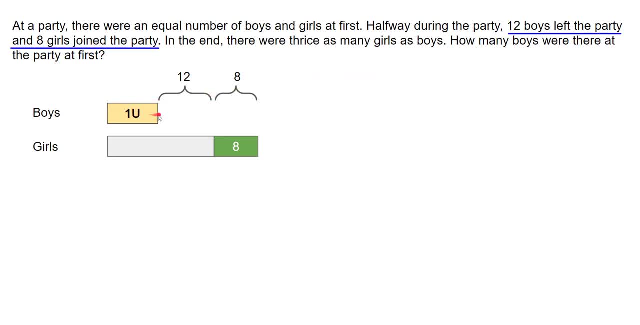 times the number of boys, Assuming this is the boy that is left. So we, if we assume this to be one unit, girls should have three units here. so if this is one unit, the whole remaining here should be actually two units, because the girls should have. 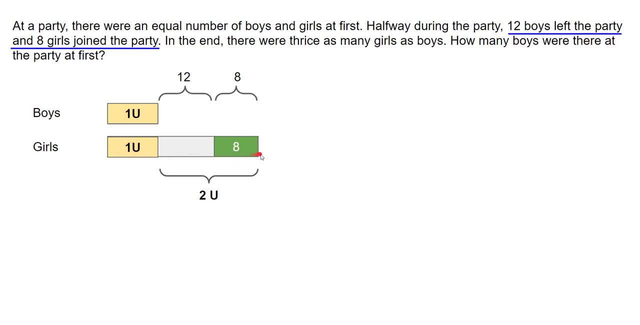 three times the number of boys. so here we should have three units, and based on the size we can very clearly see that if this is one unit, this exact size here would become one unit. so the rest of the two units will have to come out of this. 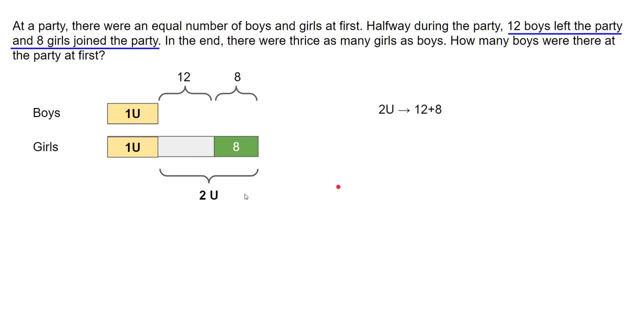 which is 12 plus 8. so we can see that two units here is equal to 12 plus 8 and that is equal to 20, and one unit represents 10 students here. now we come back to the question: how many boys were there at the party at first? the number: 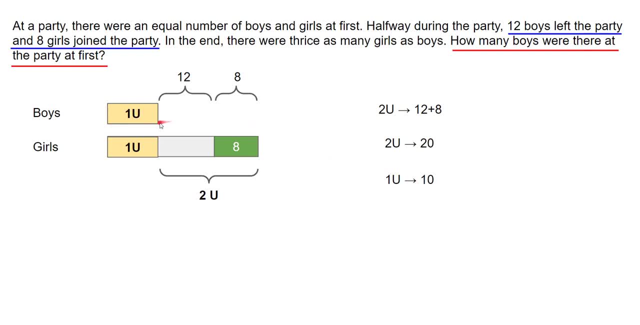 of boys at the party at first. we know that is one unit plus 12. it was up to here, right? so that's 12 plus one unit. so number of boys at first is one unit plus 12. and we know that one unit is 10 students. so here is 10 plus 12. so the number of boys at the party in 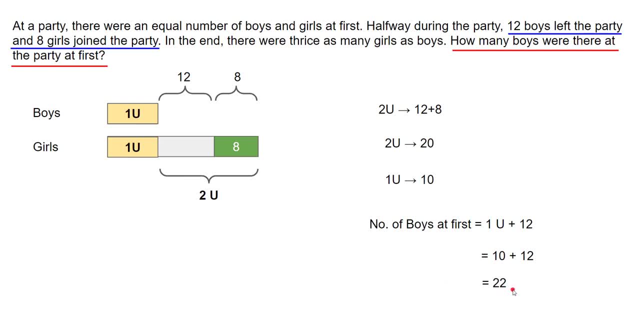 the beginning was 22. hope this is clear. this is, I would say, rather a simple question to solve using model method, and model method makes it easy to solve this kind of problem. now let's take a look at how to solve the same problem using algebra method. right, and we will also see. 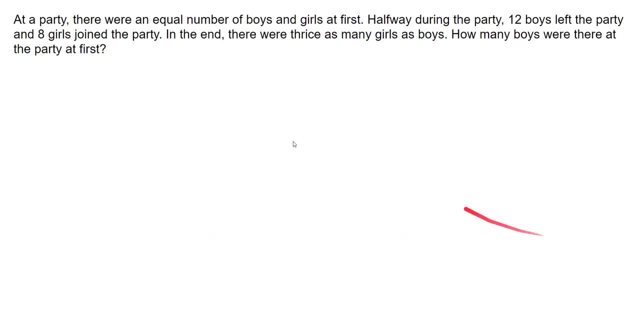 how to form equations for word problems. I'll just go through the question once again. at a party there were an equal number of boys and girls. at first halfway during the party, 12 boys left the party and 8 girls joined. in the end there were 3 times as many girls his vors. or there were thrice as many girls as spies. how? 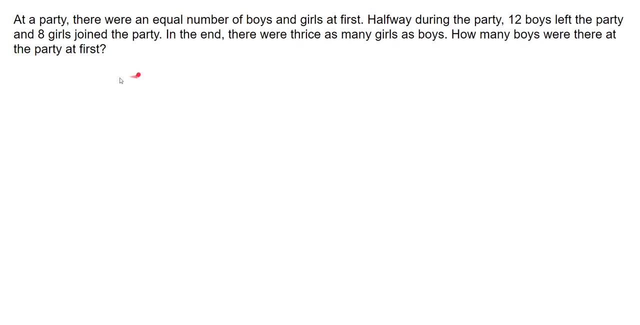 many boys were there at the party, you first. so, as we said earlier, it's we have 2 first. there are 3 distinct set of information that we have here, but first let's take the first set: of inflammation. there were an equal number of poison. girls in algebra will make an. 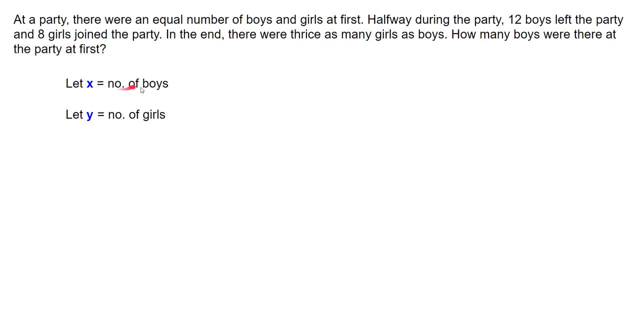 assumption saying: let X, equal to the number of boys at the party at first, and let y the number of girls in the party at first. just like the models, instead of models we are just using X and Y to denote that. so in the beginning, what happens? there were an equal number of boys and girls, right? so we know that X. 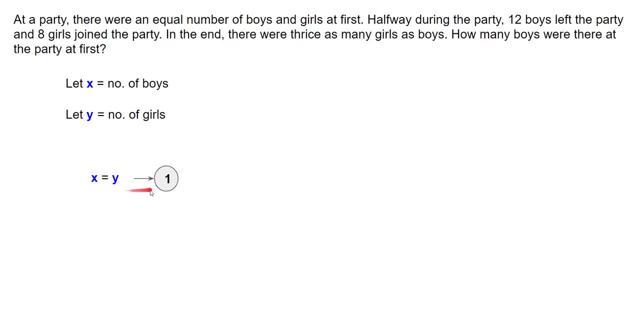 is equal to Y, so that is equation number one for us. then what happened? 12 boys left, which means the number remaining number of boys would be X minus 12, and 8 girls joined the party, so the girls remaining would increase, meaning Y plus 8. after this increase in the girls in direction and the boys, the number of 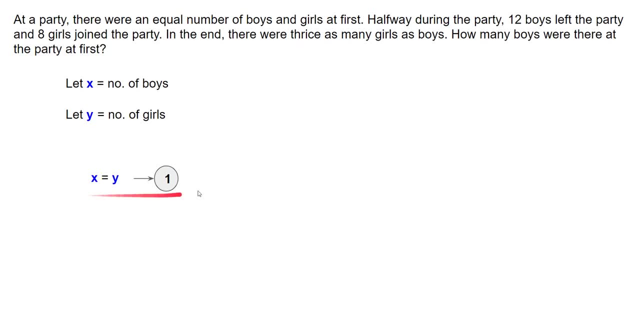 girls left became three times the number of boys. so for Y, we know the number of girls left is negative. so Y plus 8 is the number of girls left. so the number of girls left is the number of boys left. so for Y, we know that y becomes y plus 8 and this number of girls here is equal to three times the number of boys. 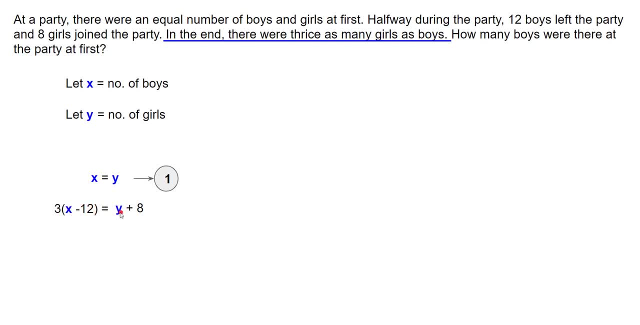 left. the number of boys left is X minus 12, and this amount is three times that. so that is our second equation. now we have formed two equations. we have to solve these equation. one simple method is called substitution method, whereby we substitute the value from one equation to another. we know 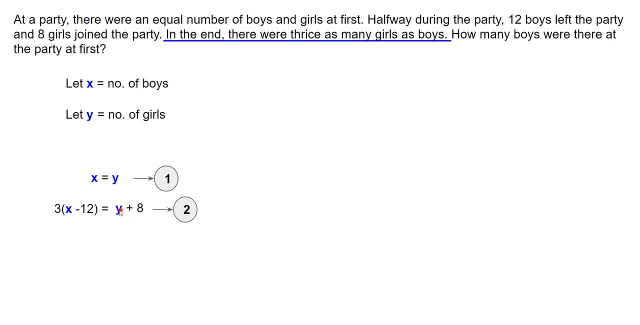 that Y is equal to X, which means here y can be replaced with X. so substituting the value of Y from equation 1 in equation 2, what happens? instead of this Y we will have X three times X minus 12 equals y plus 8, and that Y is equal to X. so b substitute X here and we multiply this. three times X gives us a value of 3.5, so we plane thatowie this: three times X gives us a Y plus 8. here we have 3 times three times 12 equals one times we have b times F is equal to x. 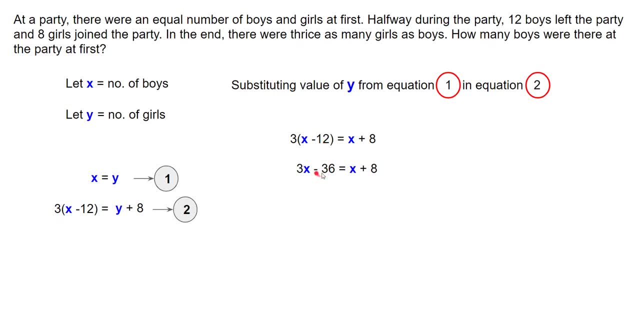 so we substitute x here. when we multiply this three times X gives us a value of 0.5, thatH, and this 3x and 3 times 12 gives you 36. so 3x minus 36 equals X plus 8. whenever we 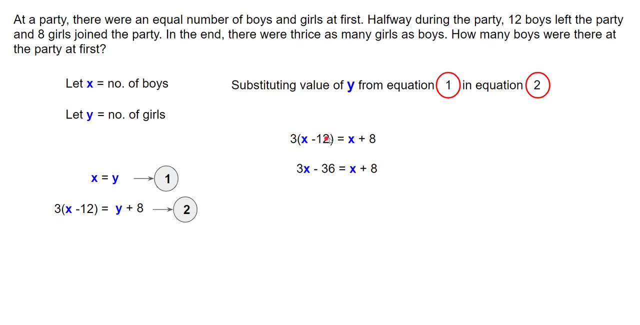 multiply. we multiply with each of the individual elements inside the brackets here. so 3x minus 12 is equal to X plus 8. and in any equation we can do operations like addition, subtraction, multiplication and division on both sides, as long as the equality is not affected. so we know that if we add both sides with the same 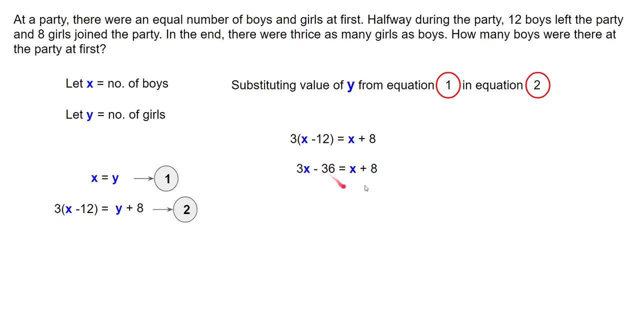 number or subtract both sides, multiply or divide both sides with the same quantity or number, the equality holds good. so we are now going to get rid of this X, so we can multiply both. sorry, we can. we can subtract both sides by X. so that means 3x minus X would become 2x. 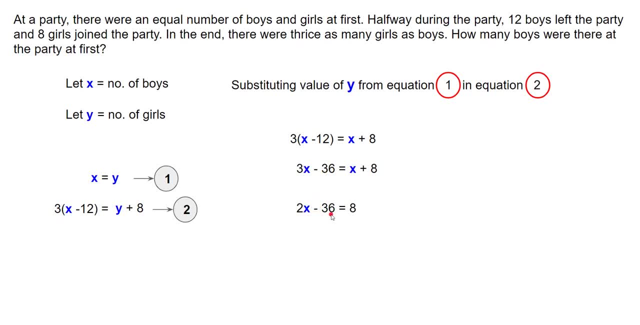 so we can subtract both sides by X. so that means 3x minus X would become 2x. this remains as it is. minus 6, 36 is equal to an X minus X cancels out, so remaining is 8. so 2x minus 36 is equal to 8. and then we want to remove this 36. 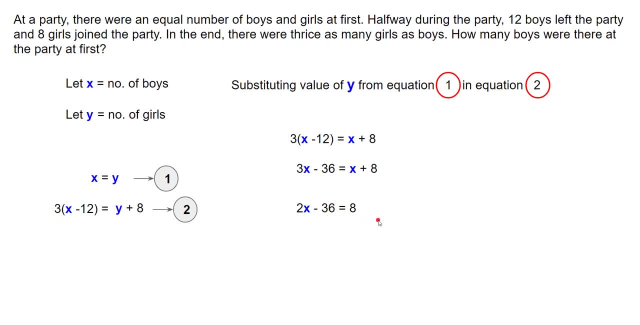 here. so what we could do is add 36 on both sides, which means minus 36 plus 36 gets cancelled out and you have additional 36 over here, so that will become: 2x is equal to 8 plus 36 and 2x is equal to 44, which means X is equal to 22. now the question says how.